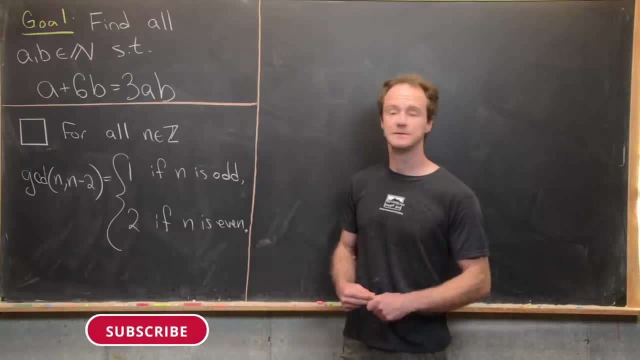 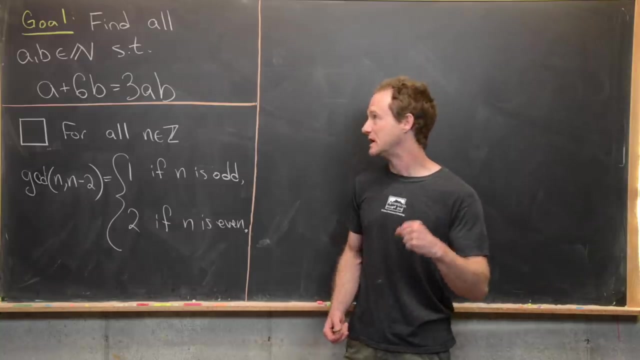 Here we're going to solve a nice little equation over the natural numbers. So our goal is to find all natural numbers, a and b, satisfying the equation. a plus 6b equals 3ab. So if you consider 0 to be a natural number, then a equals b equals 0. 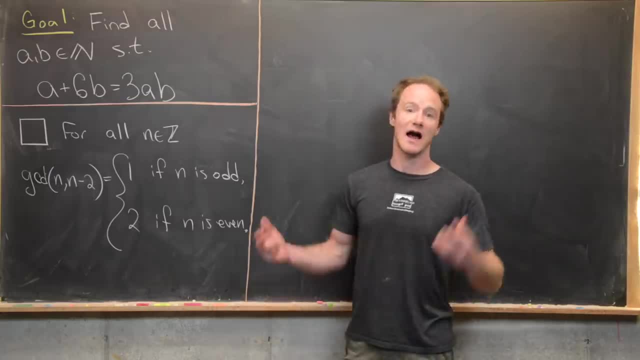 is clearly a solution to this. So we will either not include 0 as a natural number or look for all solutions that are not equal to 0.. We're going to use the following tool from elementary number theory, which we will prove So for all. 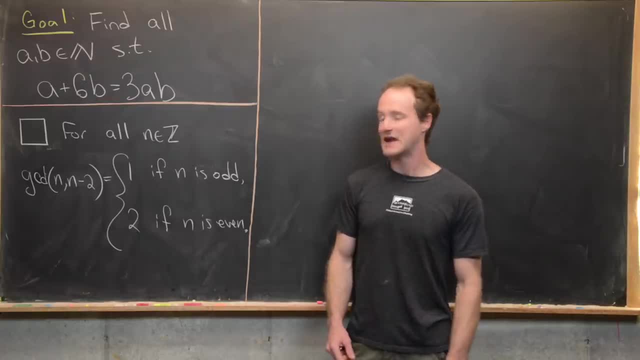 integers n. the GCD of n and n minus 2 is 1 if n is odd and it's 2 if n is even. So, obviously, if n is even, then n minus 2 is even, which means that 2 must divide both of those, But if they're odd, then these things are co-prime. Okay, so let's 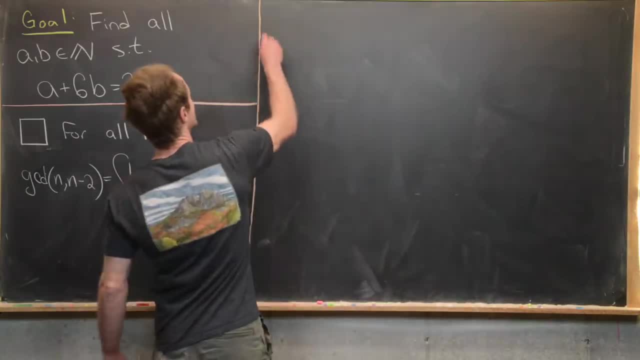 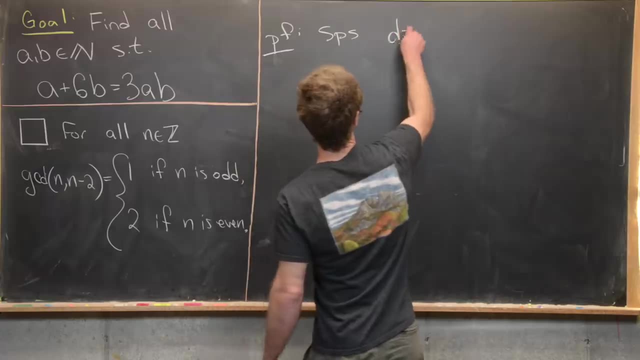 go ahead and look at this. So the proof of this is that if n is odd, then n minus 2 is even So. if n is odd, then n minus 2 is even So. the proof of this tool is fairly simple. It goes like this: So let's suppose that d equals the. 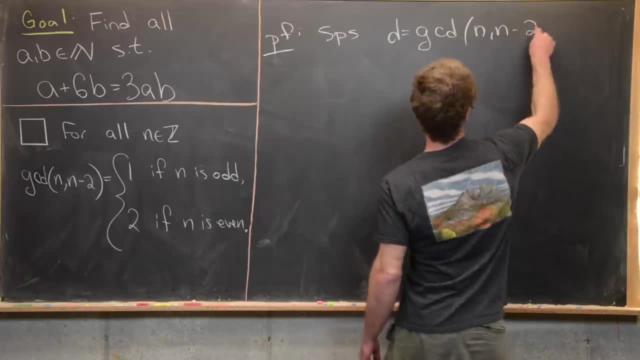 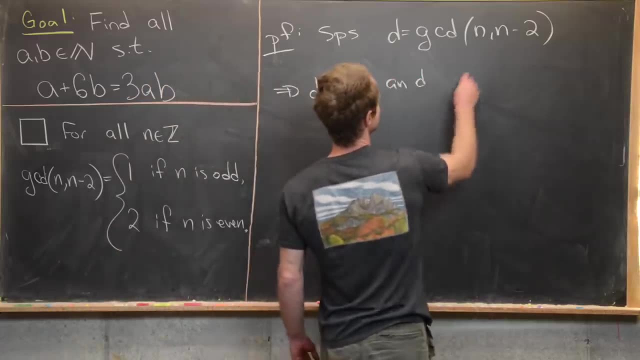 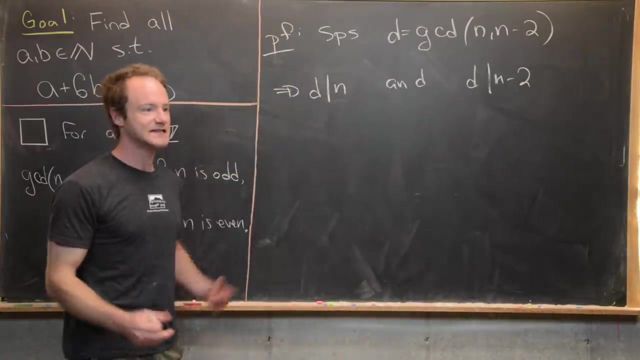 GCD of n and n minus 2.. So now that tells us that d divides n and d divides n minus 2.. And I should say that I'm doing maybe a few steps here that I wouldn't really need to do if I had done all the work. that would happen in an 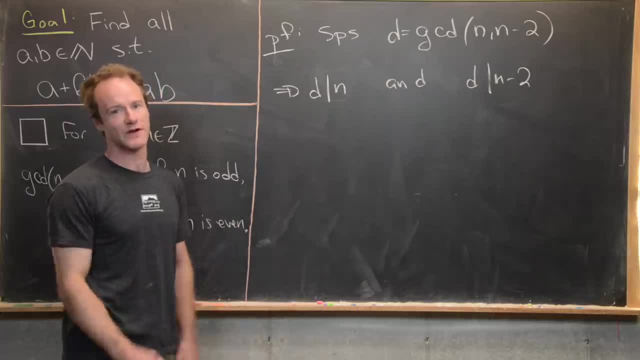 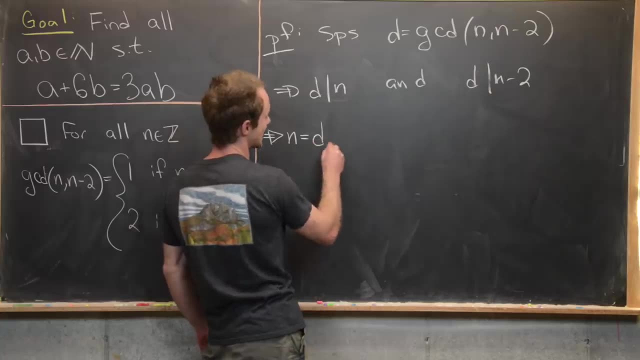 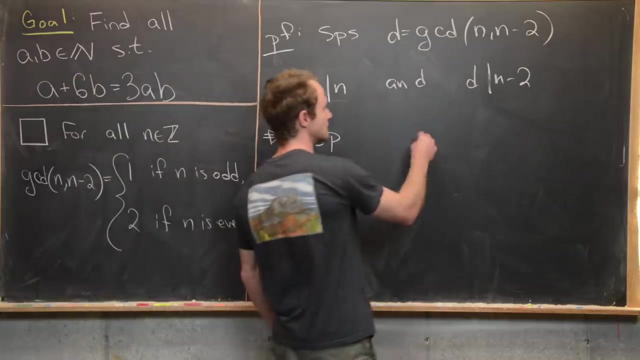 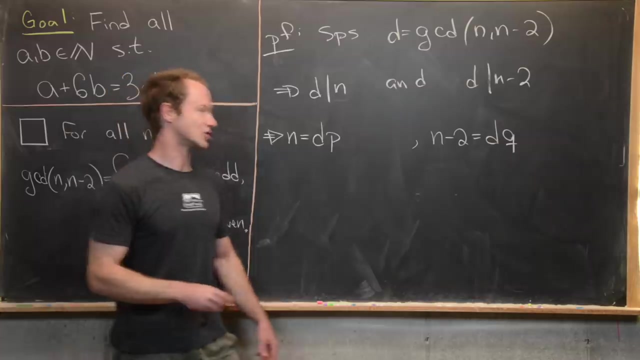 elementary number theory. But just to be thorough, we're going to do a couple of extra steps here. So the fact that d divides n, that means n equals d times p for some natural number p. And the fact that d divides n minus 2, that means that n minus 2 equals d times q for some, and I should say integer q here. So 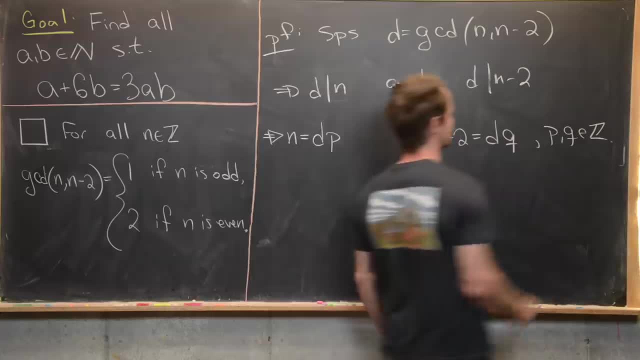 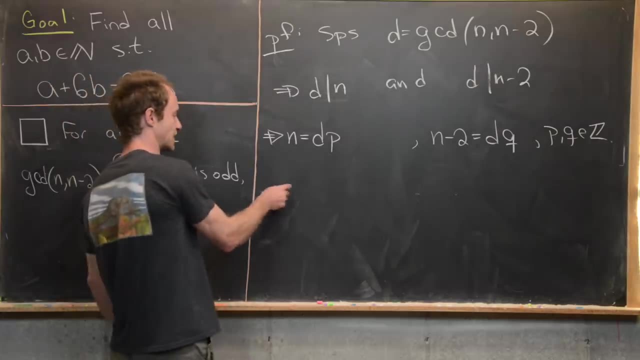 here we have. p and q are integers, because in this case we're working over the integers. Great. Now the next thing that I want to do is subtract these two equations from each other in order to get like kind of too isolated. So we'll do this equation. 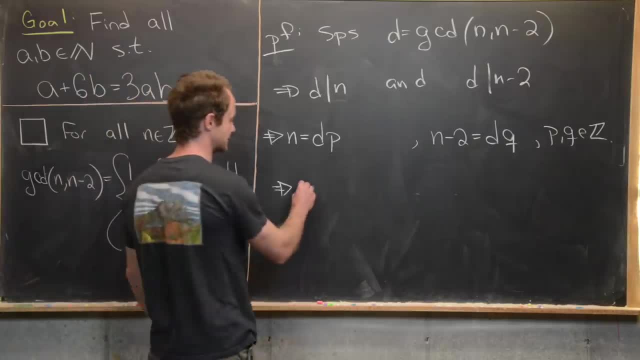 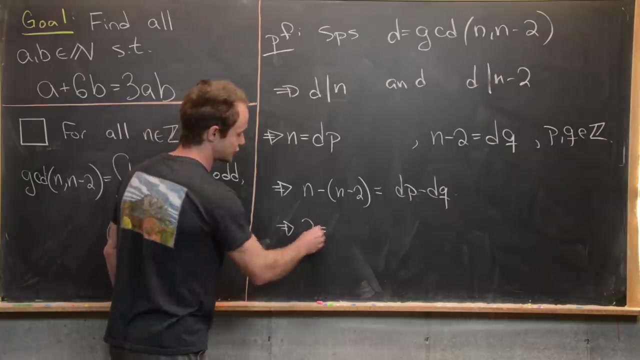 minus this equation. So let's see what that gives us. We have n minus n minus 2. so that's the difference of the left-hand side of these equations equals dp minus dq. But now notice, simplifying this left-hand side gives us 2, even if 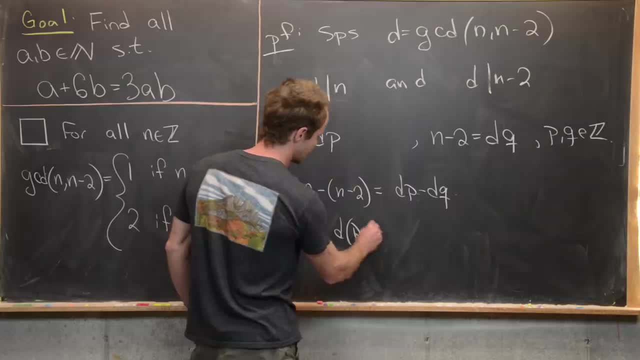 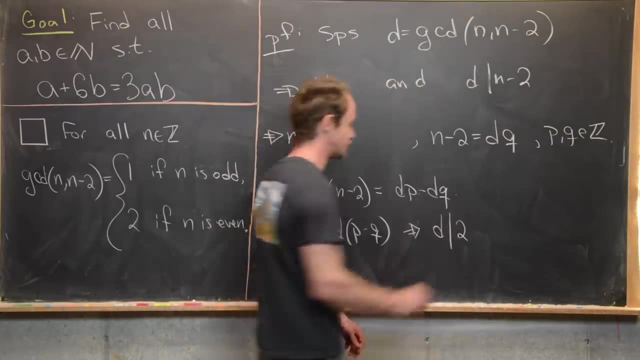 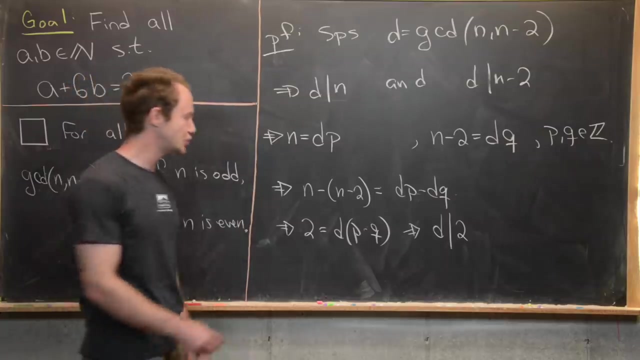 this equals d times the quantity p minus q. but now reading this off, we see that d divides two. in other words, the greatest common divisor of these two numbers must divide the number two. but since two is prime, that only gives us two possibilities for d. so that tells us that d 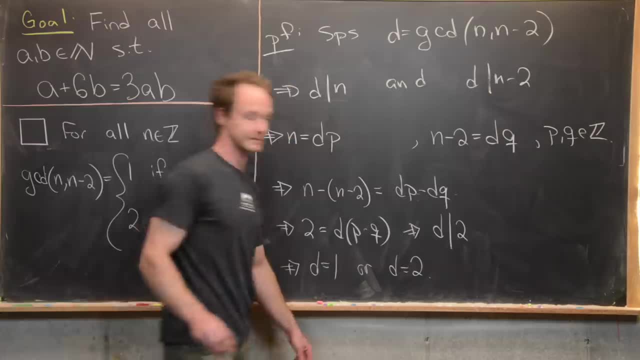 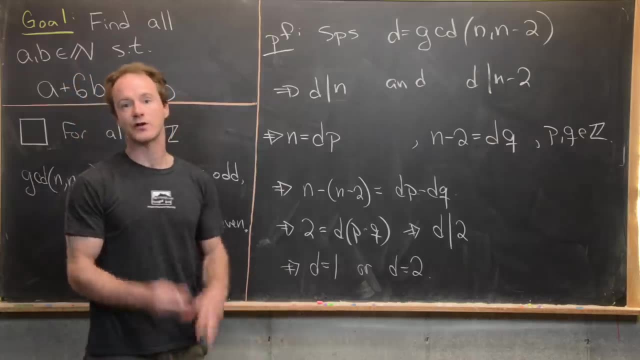 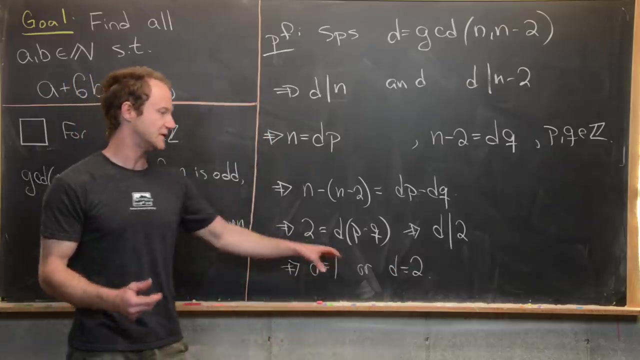 equals one or d equals two. and now we're essentially done. so. if n is even, then n minus two is even, so they're automatically both divisible by two, and in fact they can't be divisible by anything bigger than two because of what we've shown here. and then, if n is odd, 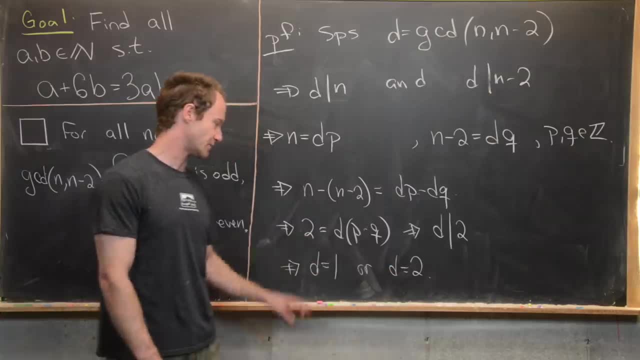 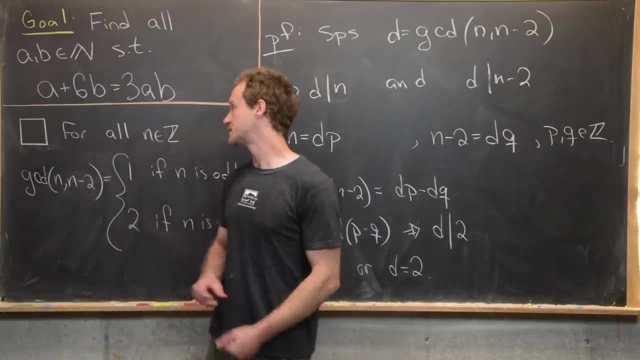 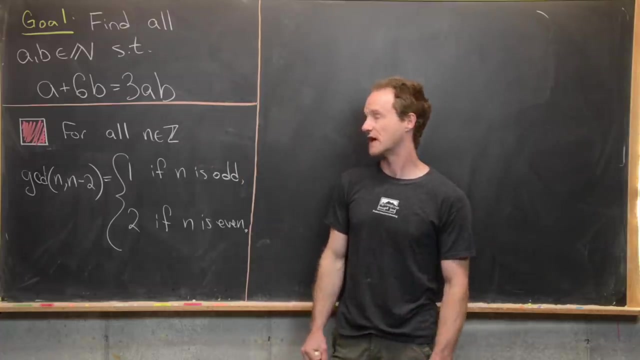 then n minus two is odd, and so they cannot be divisible by two, which means they're only divisible by one, and that makes one their gcd. okay. so we've proved this tool, and now we're going to move on to our main objective, in other words solving this equation among the natural numbers: a plus 6b equals 3ab, so the first thing that we're 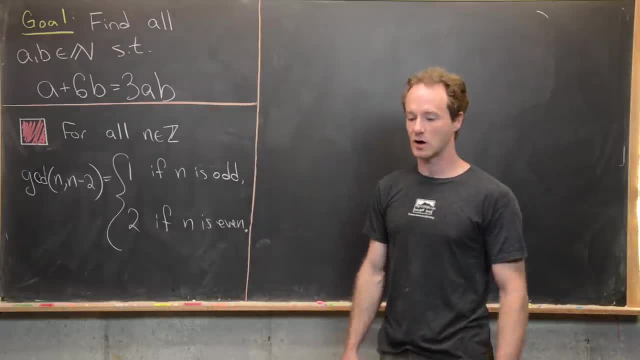 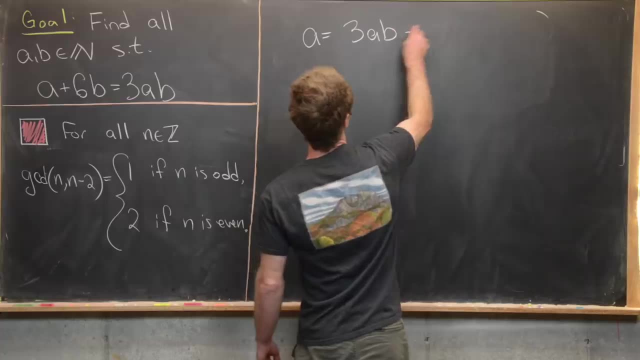 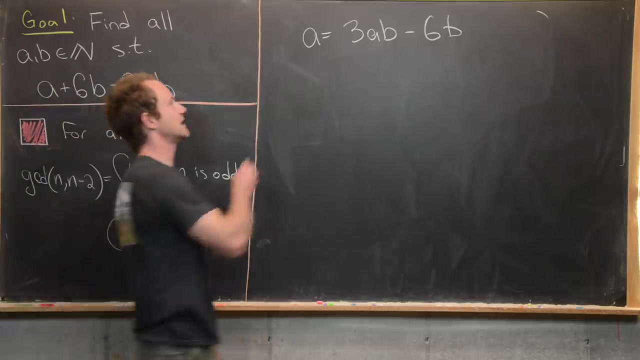 going to do is rewrite this guy so that all of the b's are on one side of the equation. so let's go ahead and do that. we have a equals 3ab minus 6b. okay, good, now we can take a greatest common factor out of that right hand side. 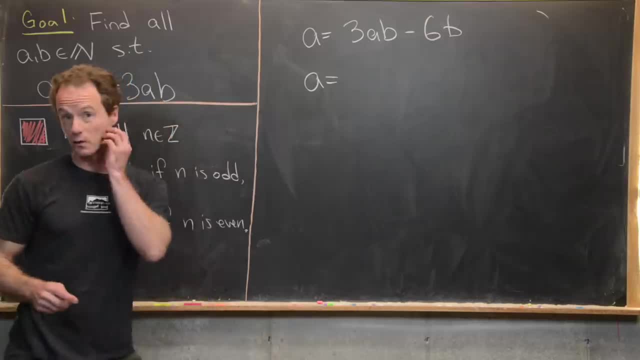 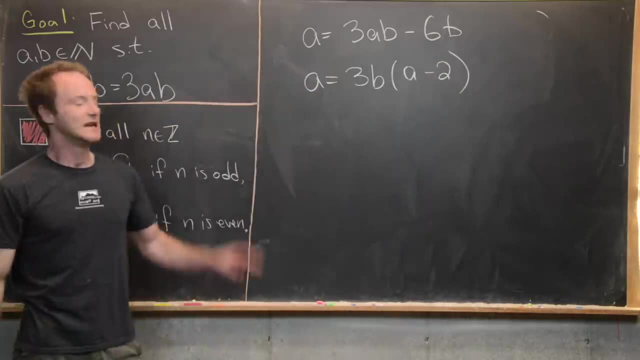 you. let's see what that gives us. so the greatest common factor here will be 3b, so we have a equals 3b times a minus 2. now we want to use our tool, and since our tool has two cases here, if n is odd, 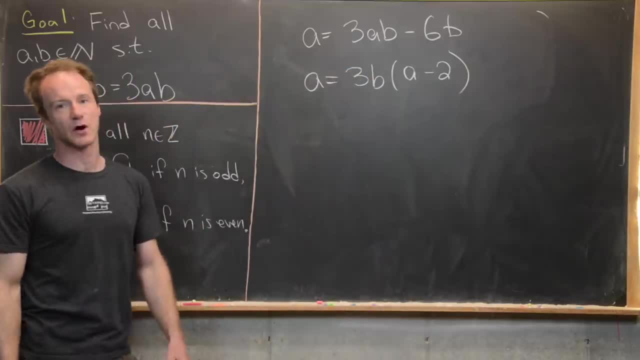 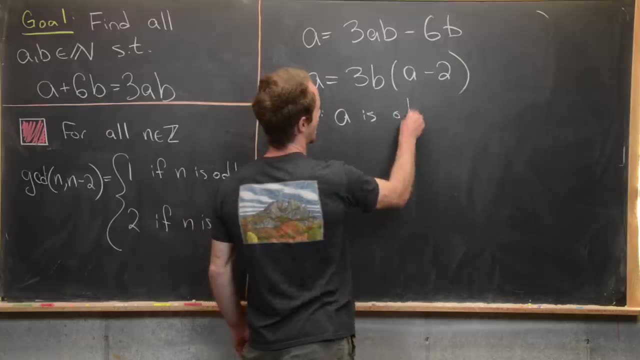 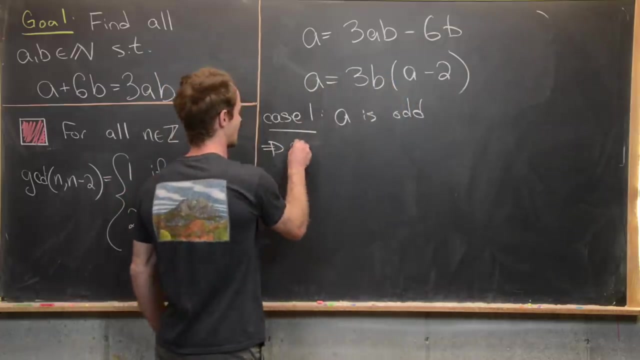 and n is even. that means we're going to need to break this apart into two cases, so let's go ahead and do that. so case number one is: a is odd. great, but now if a is odd, just like we showed over here, we have the gcd of a and a minus 2 is 1. in other words, these are: 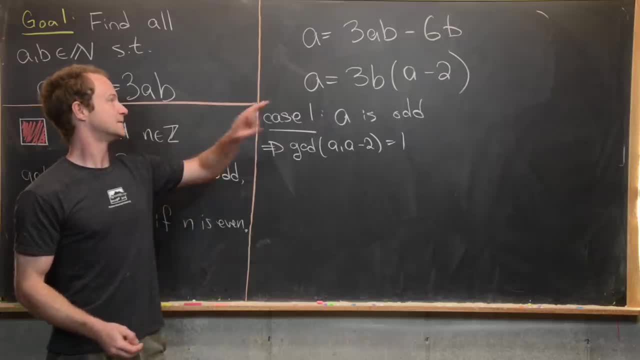 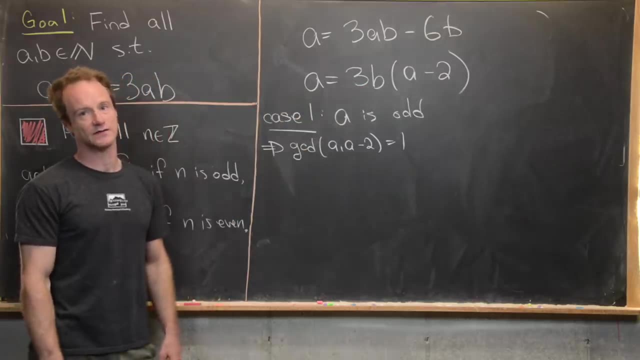 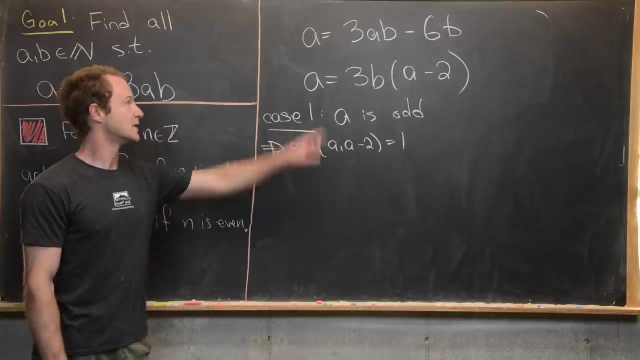 co-prime. but what that tells us is that because a divides the left hand side of the equation, a must divide the right hand side of the equation. but because these are co-prime, a cannot divide a minus 2, which means a must divide 3b. 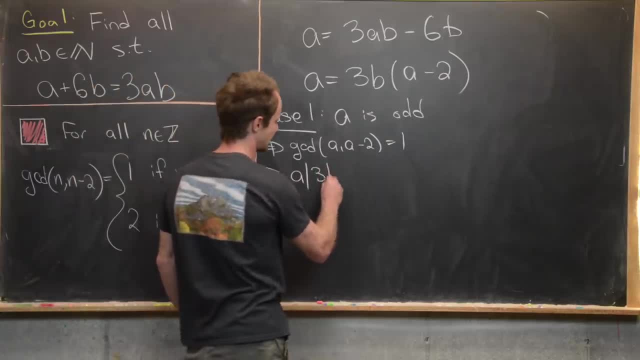 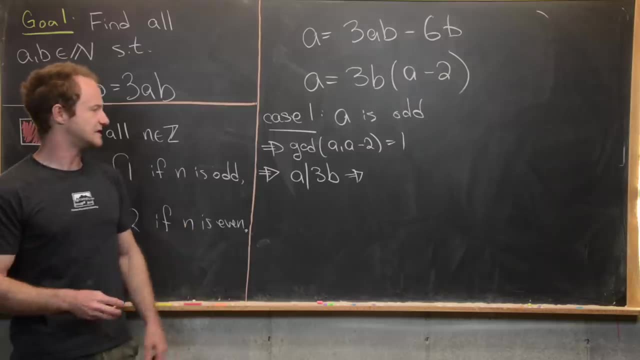 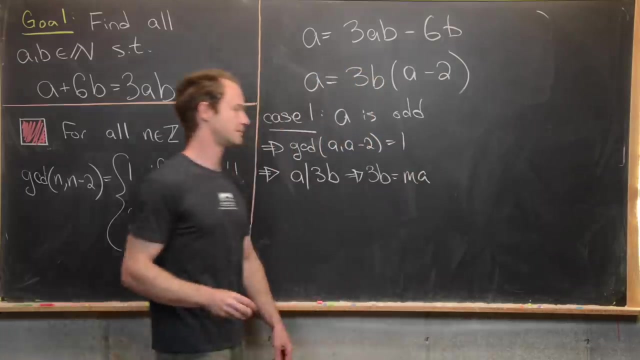 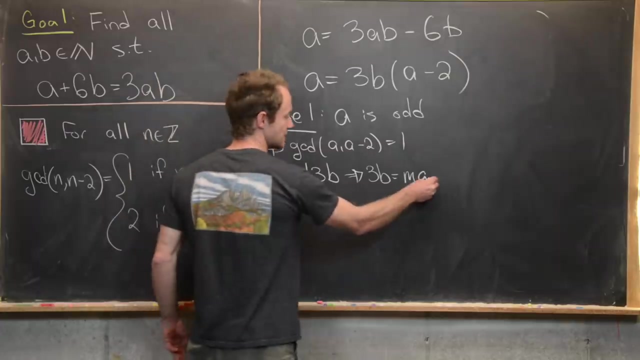 so that gives us a divides 3b. great, but now what we can do is use the definition of divisibility to say that this means 3b equals m times a, where m is just like the natural number that makes that happen. okay, good, now the next thing that we're going to do is take this result and insert it. 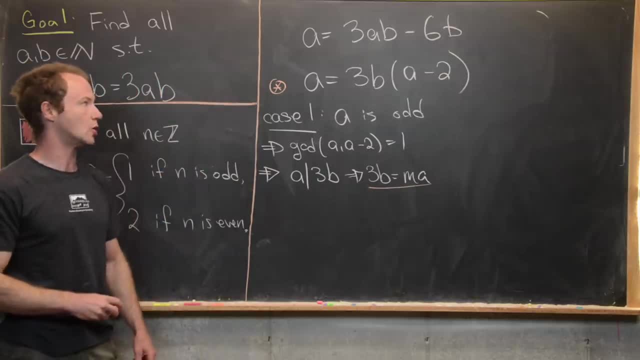 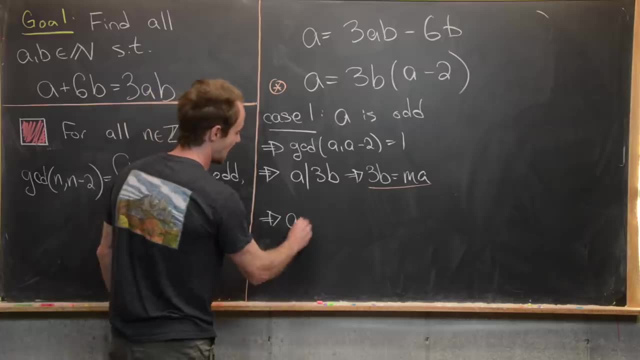 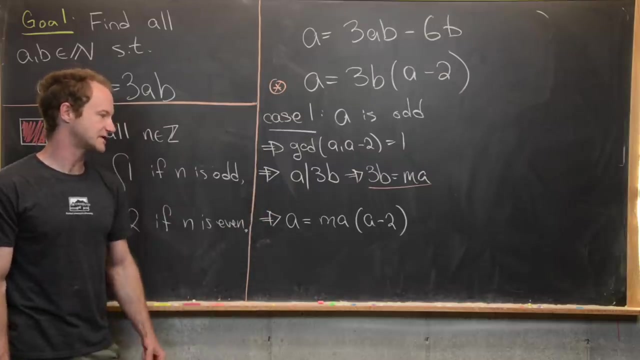 up here into this equivalent equation, and we're going to do that by dividing it by m. So again to our goal and see what that gives us. So we'll replace 3b with m times a, So that gives us a equals m times a times a minus 2.. Now we can go ahead and cancel a from both sides of the equation. 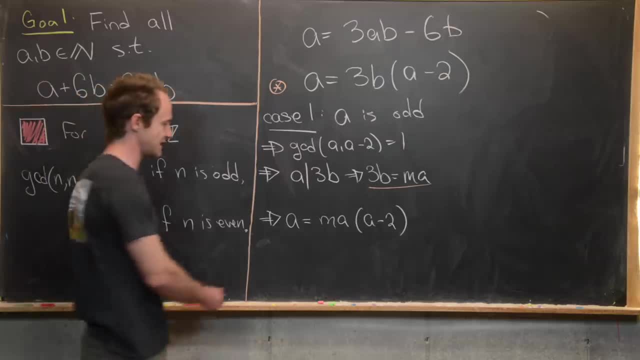 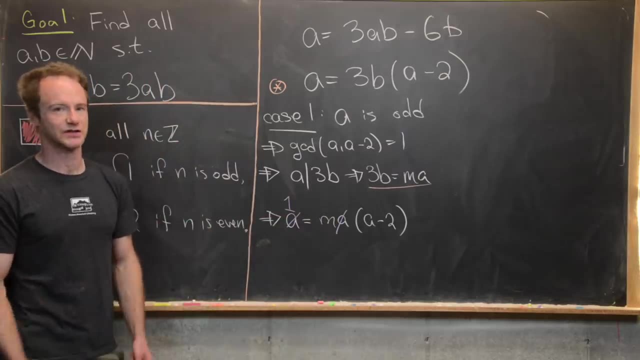 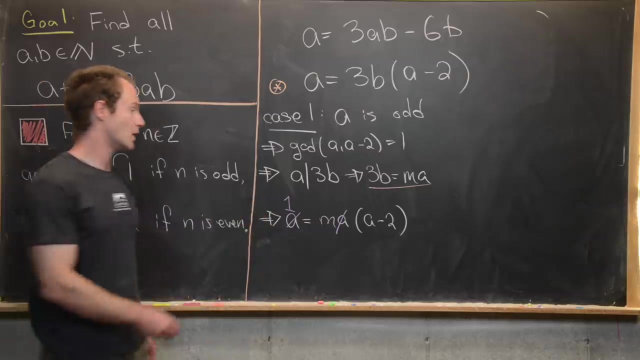 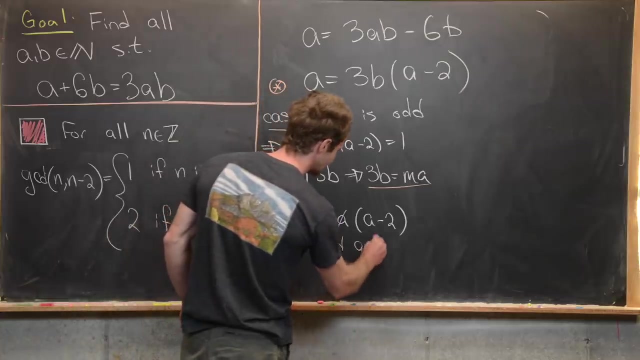 because we've already discussed that a is not equal to 0 in this setup. So if we cancel here, we're left with the number 1.. If we cancel here, we're left with m times a minus 2.. So we have 1 equals m times a minus 2.. But what that tells us is that m equals 1 and a minus 2 equals 1.. 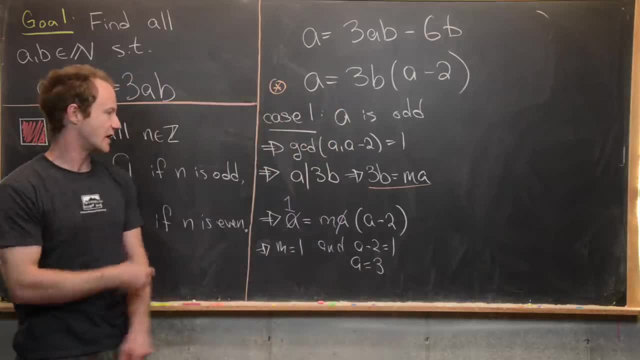 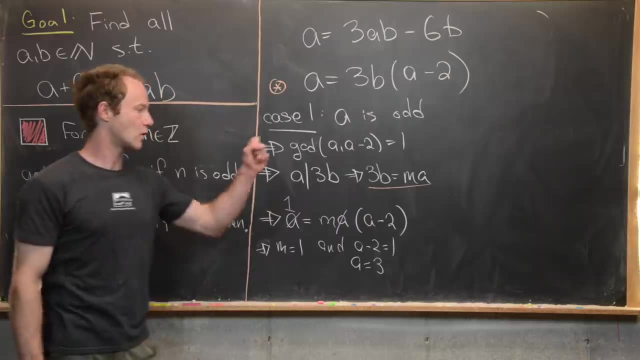 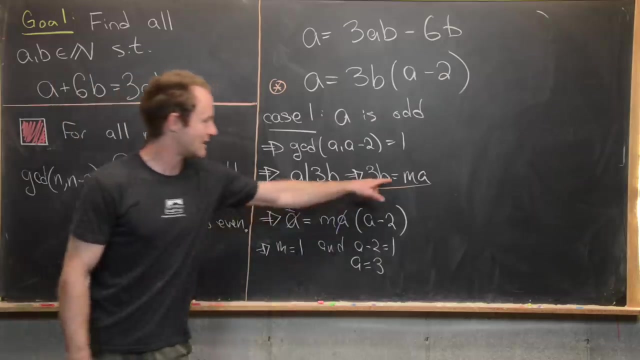 In other words, a equals 3.. Let's talk our way through that. So we know that a is is a natural number, which tells us that it is 1 or larger. And then, since it's 1 or larger and b is also a natural number, that makes m a natural number. But if m is a natural number, it's 1 or 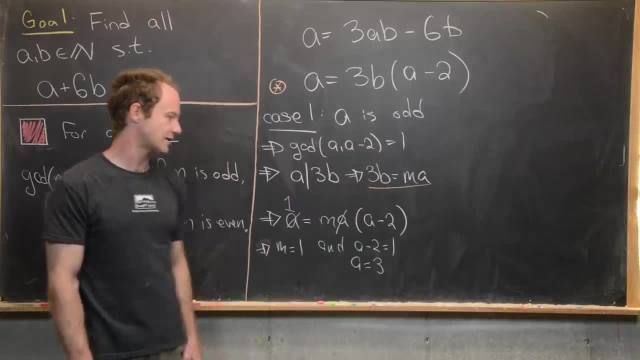 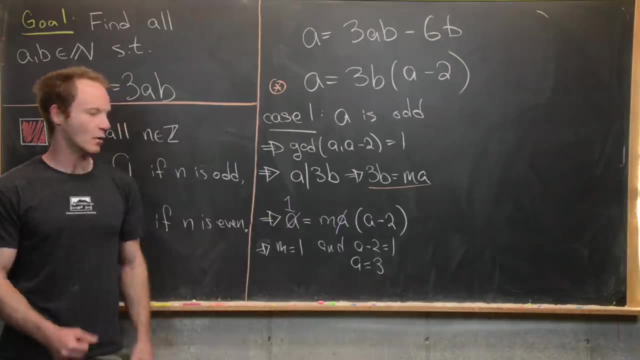 larger. So this bit is positive, which means this bit also has to be positive, which means they both have to be 1, because those are the only two natural numbers that you can multiply to get 1, which is on the left hand side. So now, if we've got a equals 3 and m equals 1, we can go ahead. 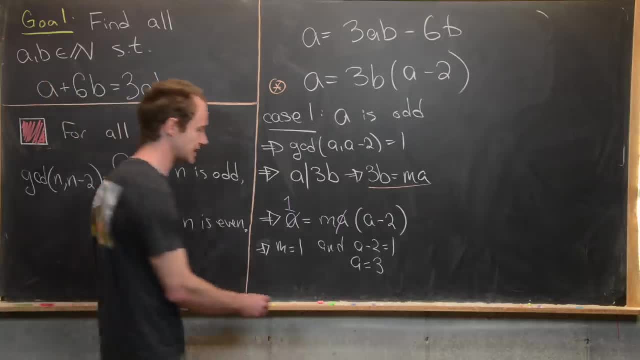 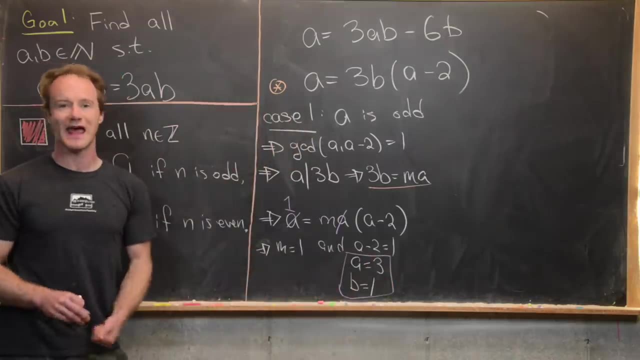 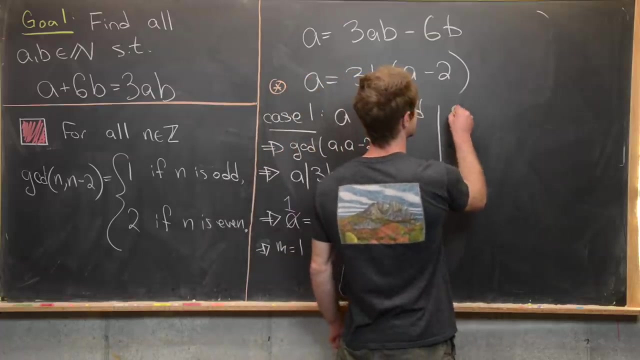 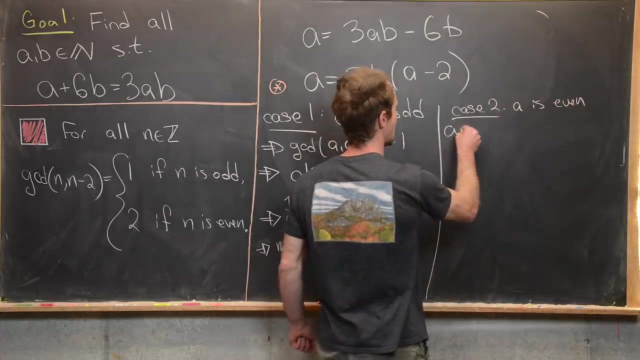 and plug that up here, and that gives us 3b equals 3.. In other words, b equals 1.. And that is our only solution, under the assumption that a is odd. Now I'll move on to the next case, which is if a is even. So let's go ahead and do that. So, case 2: a is even, and here I'll write a. 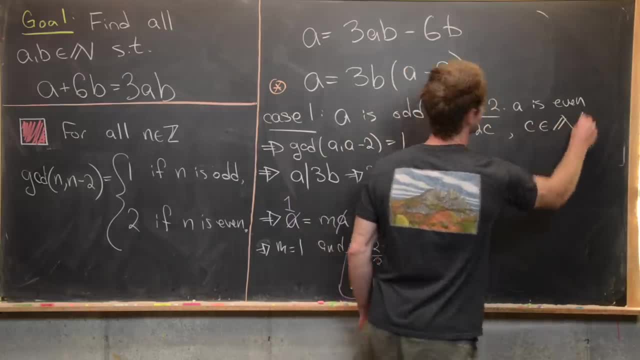 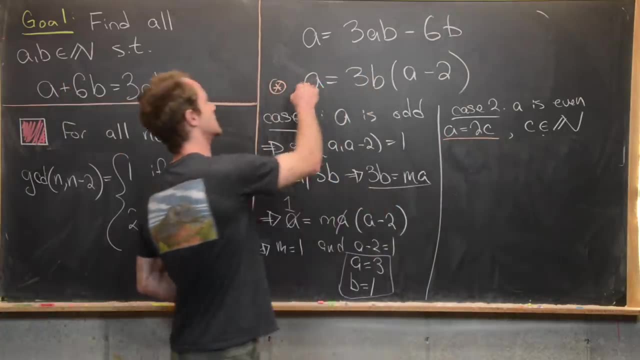 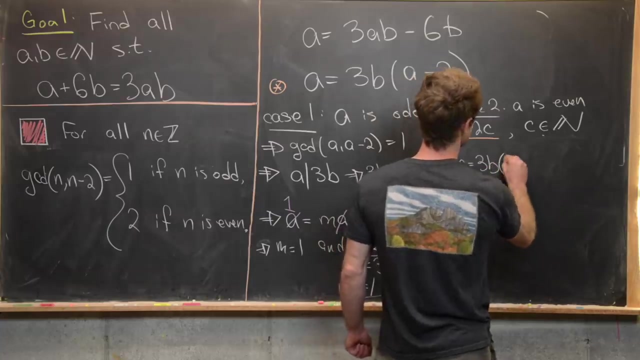 equals 2c, where c is some natural number. Okay, fantastic. But now, just like we did before, we'll insert this equation back into our original setup. So here we have 2c equals 3b times 2c minus 2.. Okay, good, Now we can like. 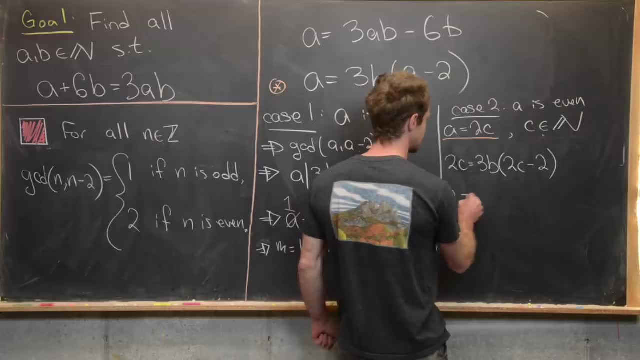 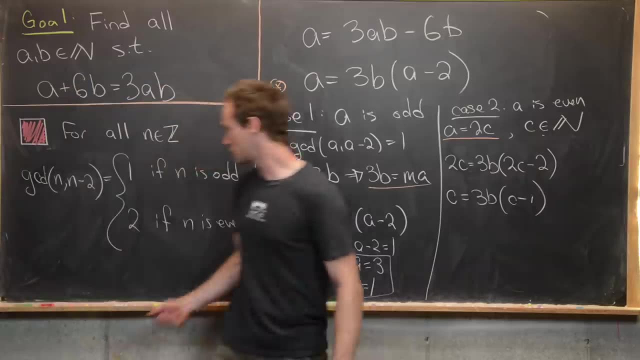 divide both sides by 2 and that's going to give us c equals 3b times c minus 1.. And now our result, which is very, very similar to this, shows that the gcd of n and n minus 1 is always equal to 1.. 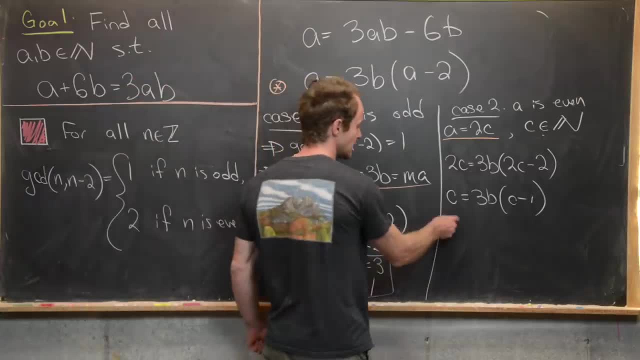 So, by the same argument, we have: a: 2c equals 3b times 2c minus 1.. And now our result, which is very, very similar to this, had over. here we see that since c divides the left hand side of the equation, it must divide the. 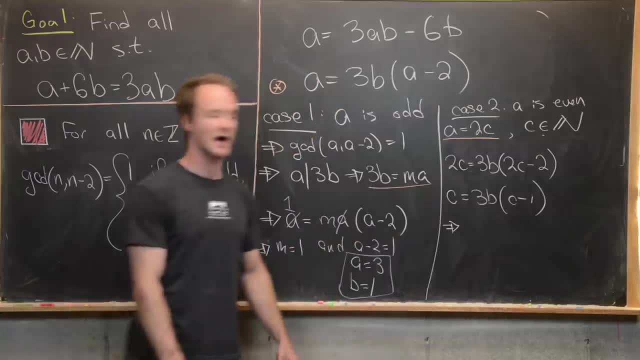 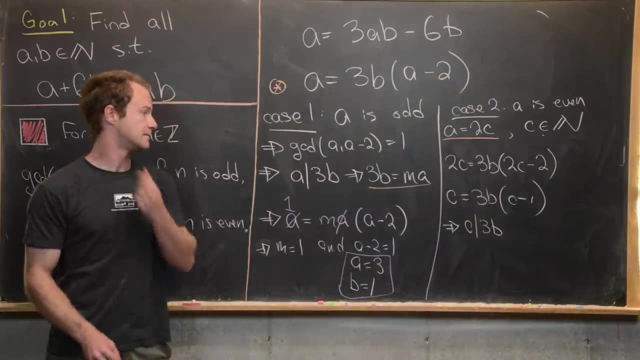 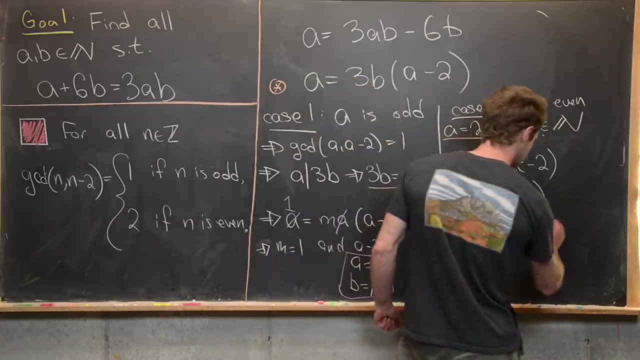 right hand side of the equation. And then, since it is co-prime, with c minus 1, we know that c must divide 3b. Great, But now from here we can say immediately that 3b equals n times c, Just like. 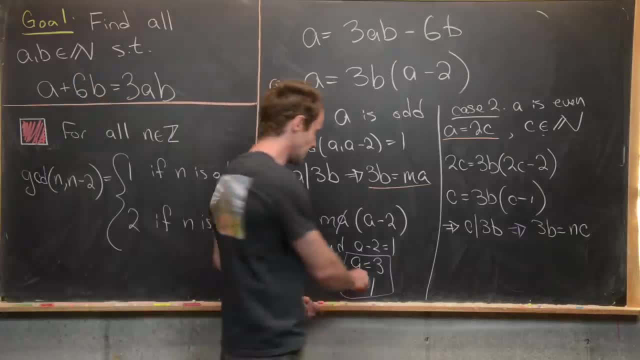 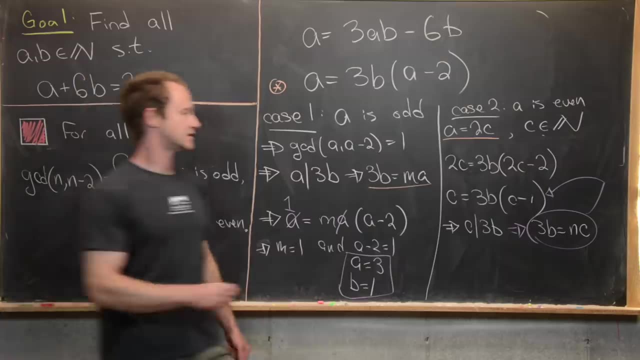 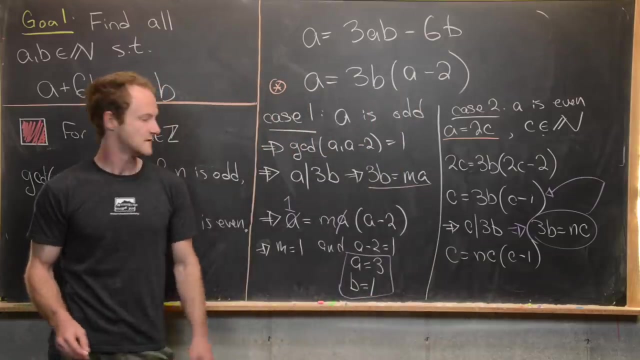 we did right here. Now what we'll do is go ahead and take this and plug it back into the equation which is right above. so that's gonna give us c equals n times c times c minus 1. but now we can cancel the c's from both sides of the equation, like kind of for the same reason that we 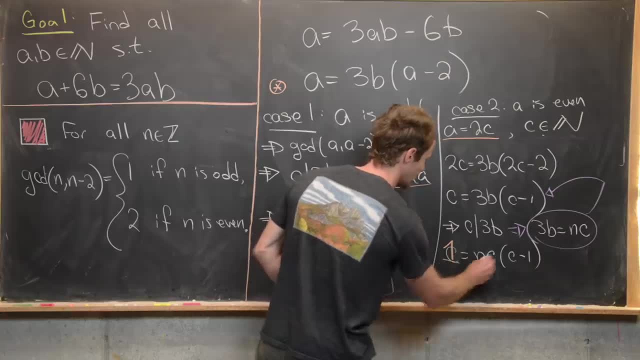 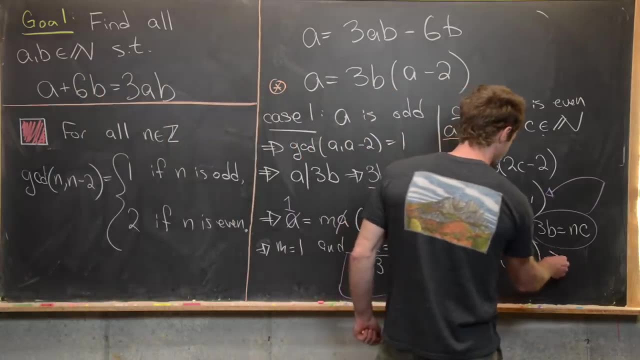 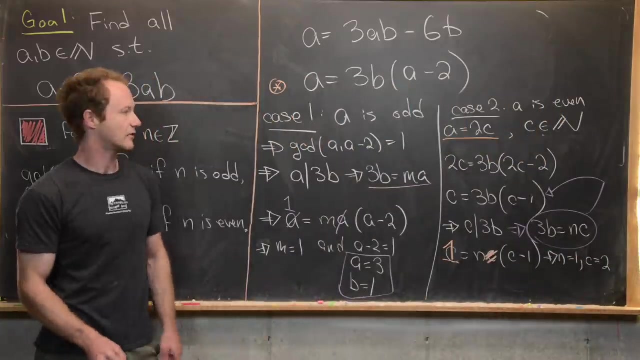 did before, and that's going to leave us with a 1 on the left-hand side. That'll leave us with n times c minus 1 on the right hand side, but the only natural number solutions to that are n equals 1 and C equals 2.. Okay,